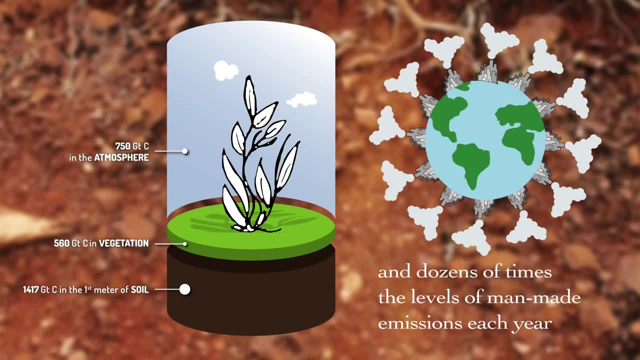 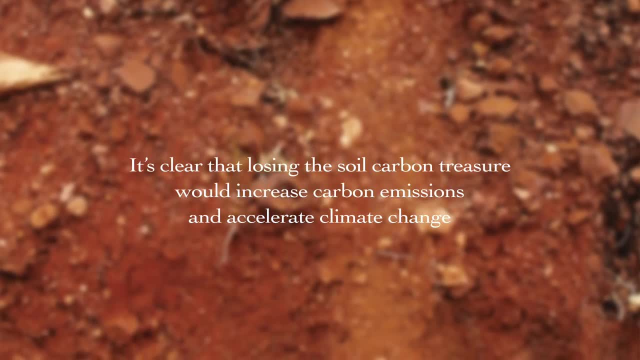 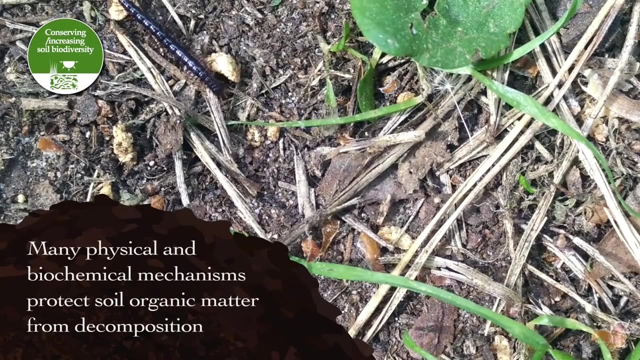 And dozens of times the levels of man-made emissions each year. It is clear that losing the soil carbon treasure would increase carbon emissions and accelerate climate change. But we can do something about it. Many physical and biochemical mechanisms protect soil organic matter from decomposition. 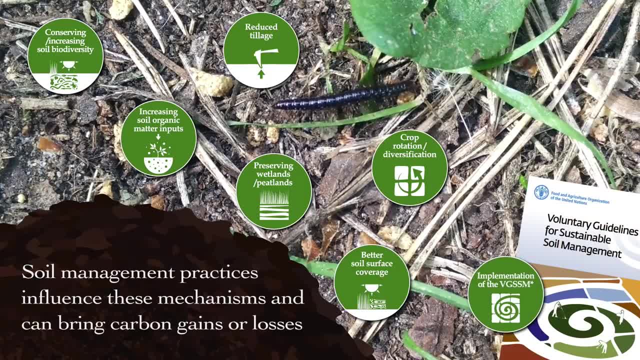 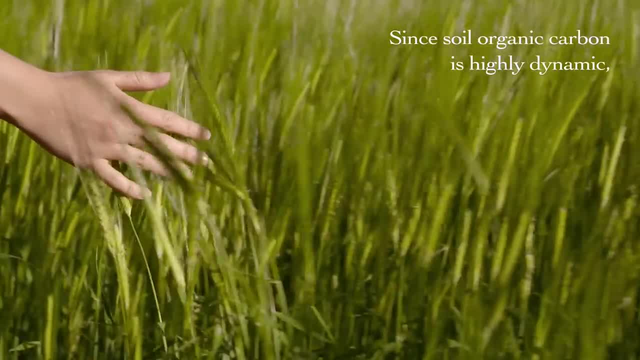 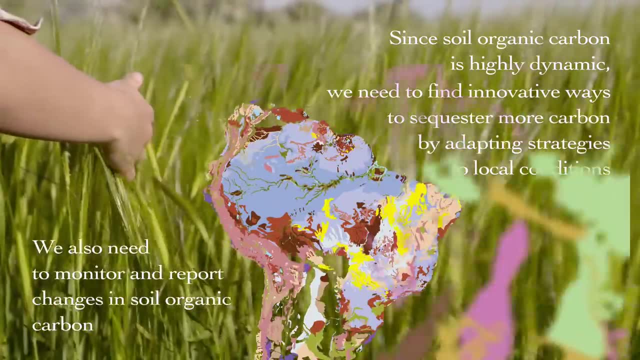 Soil management practices influence these mechanisms and can bring carbon gains or losses. Since soil organic carbon is highly dynamic, we need to find innovative ways to sequester more carbon by adapting strategies to local conditions. We also need to monitor and report changes in soil organic carbon. 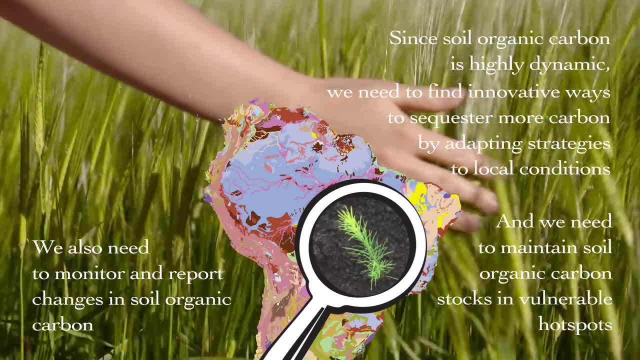 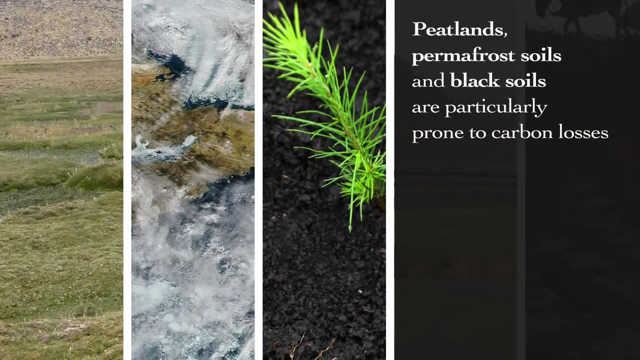 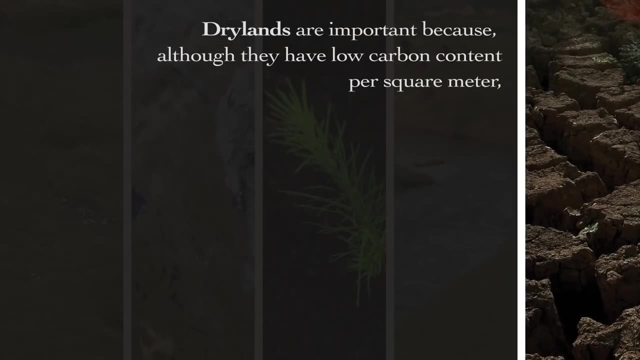 And we need to maintain soil organic carbon stocks in vulnerable hotspots. Peatlands, permafrost soils and black soils are particularly prone to carbon losses. Grasslands store more than double the amount of carbon in all other agricultural areas. Drylands are important because, although they have low carbon content per square meter, they cover a large surface area. 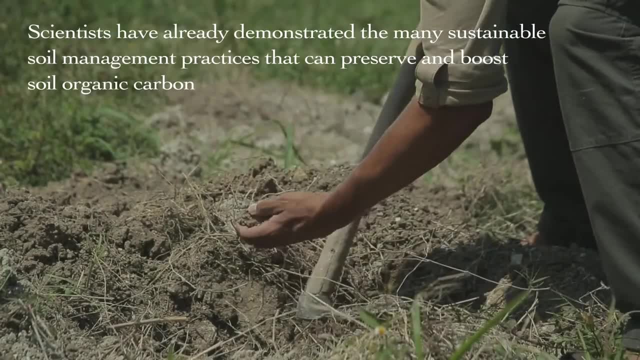 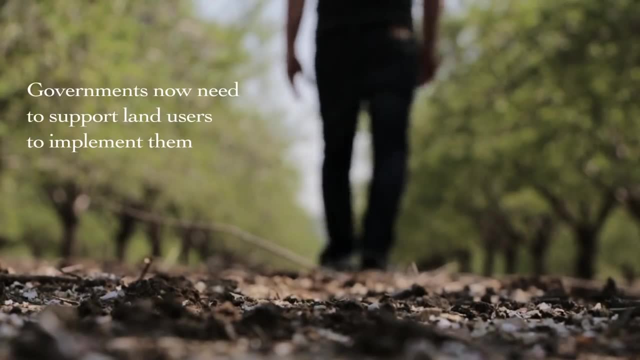 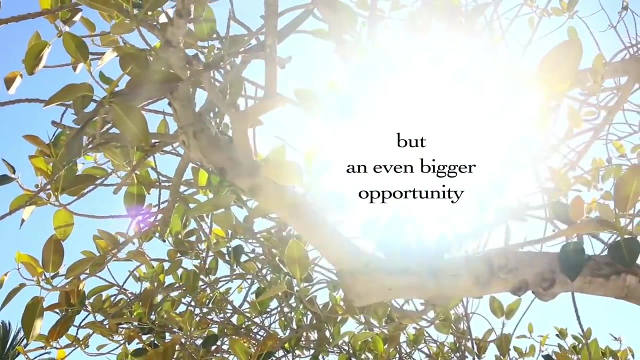 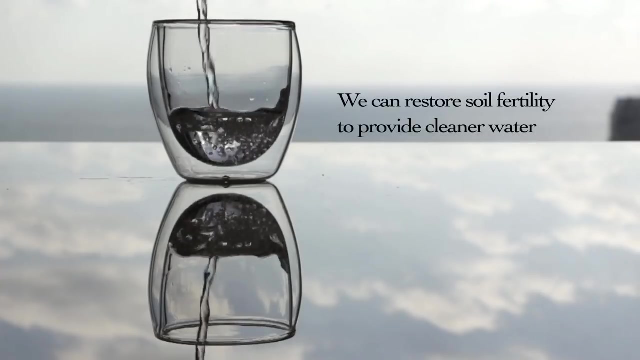 Scientists have already demonstrated the many sustainable soil management practices that can preserve and boost soil organic carbon. Governments now need to support land users to implement them. This is a huge task, But an even bigger opportunity. We can enhance resilience to extreme events. We can restore soil fertility to provide cleaner water and nutritious food. 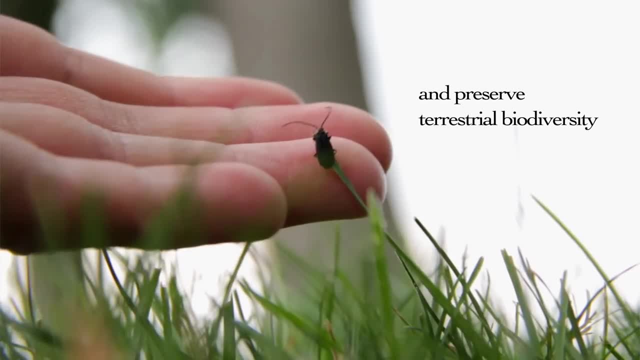 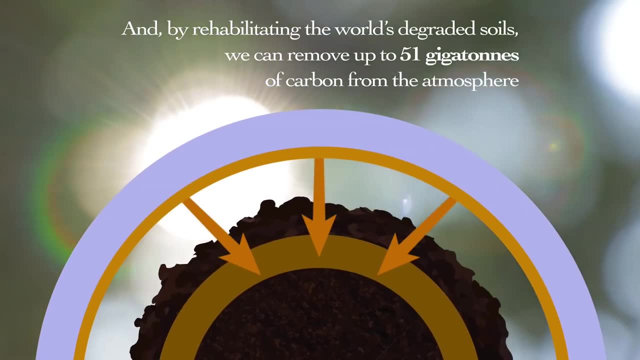 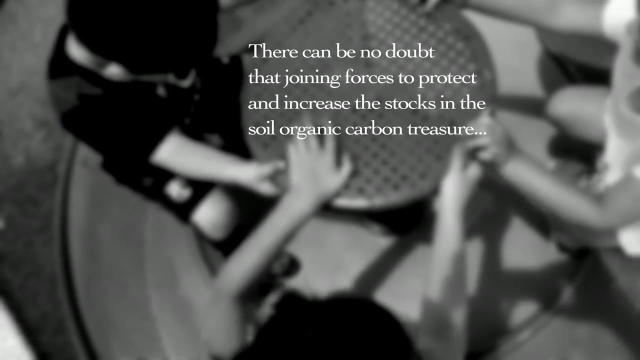 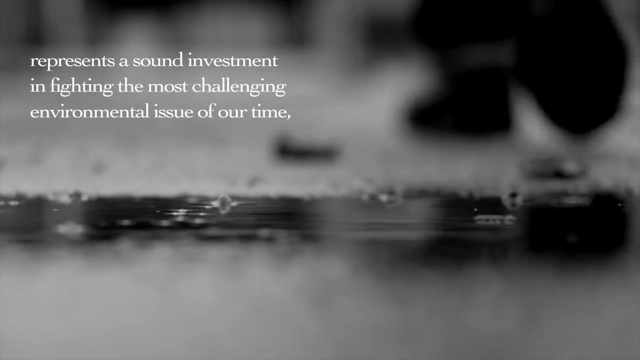 And preserve soil fertility And preserve terrestrial biodiversity, And by rehabilitating the world's degraded soils we can remove up to 51 gigatons of carbon from the atmosphere. There can be no doubt that joining forces to protect and increase the stocks in the soil organic carbon treasure represents a sound investment in fighting the most challenging environmental issue of our time.